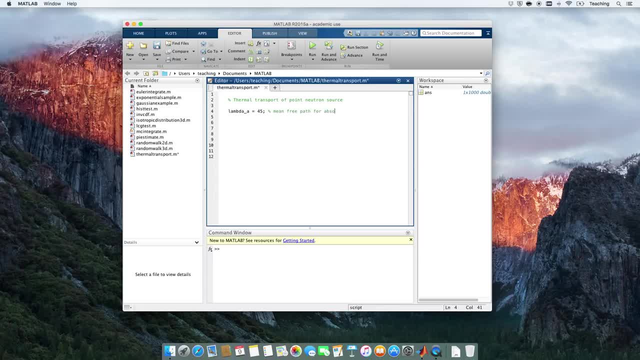 that mean free path, And we're going to use that here. So let's get the warming power of this current And we're going to call that lambda a And we're going to use CGS units, absorption, and I'm going to say that lambda s equals point three, which is the 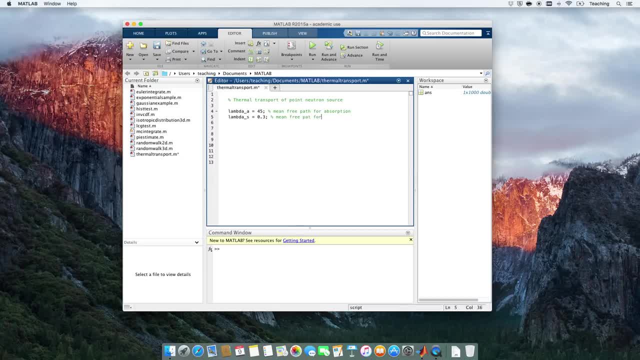 mean free path for scattering. so of course, if I only had absorption, then the neutrons, if they were, say, traveling all in one direction, would continue traveling that direction for a typical distance of 45 centimeters and then be absorbed. so we would know how the intensity would vary as a function of 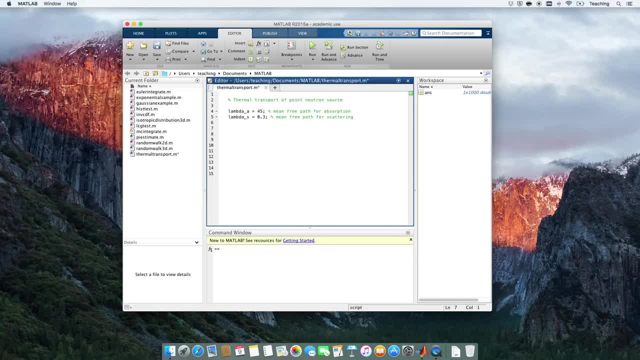 distance with an analytical calculation. but when we include scattering, things were a little bit, a little bit more difficult. now what we do to transport the neutrons is we're going to take exponentially distributed steps according to the total mean free path. so in order to calculate this, we're going 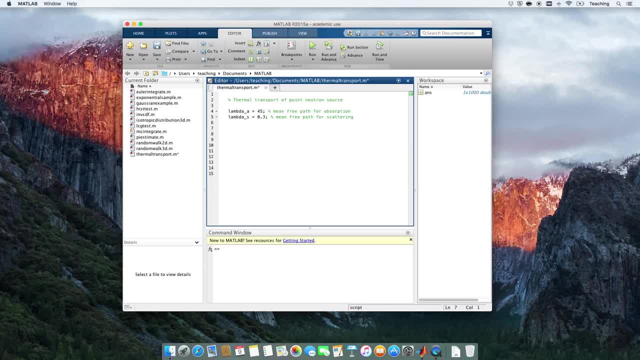 to calculate some intermediate variables. I'm going to call these are the macroscopic cross sections. so I'm going to call those: Sigma a, which is the macroscopic cross section for absorption, which is simply one over the mean free path, and Sigma s is equal to one over the mean free path. 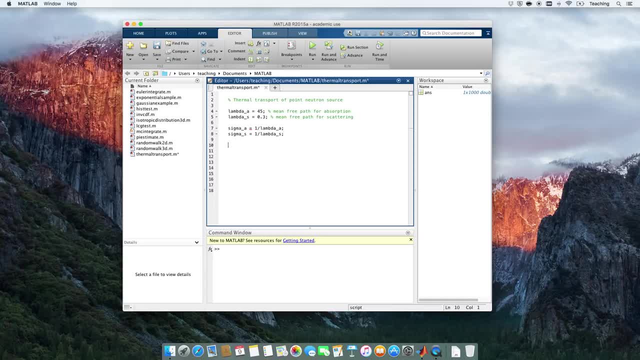 for scattering and the total cross section. I'm going to call that Sigma t- is equal to Sigma a. sigma s- and we can understand this by thinking of the those two areas as being additive and we have a probability- probability of an interaction occurring in the water molecules which is proportional to each of those two. 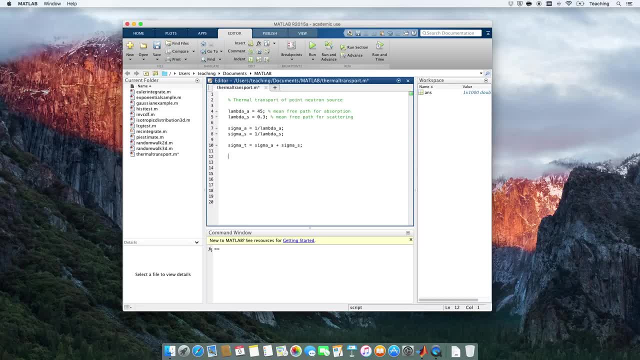 cross-sectional areas and these are the macroscopic ones. so we've multiplied implicitly by the number density of the, the water molecules in the water. now we could calculate those numbers directly by using the microscopic cross-sectional, but we're not going to do that here. so the total mean free path lambda t is: 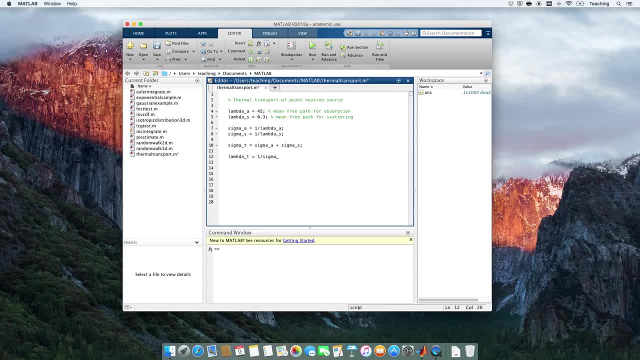 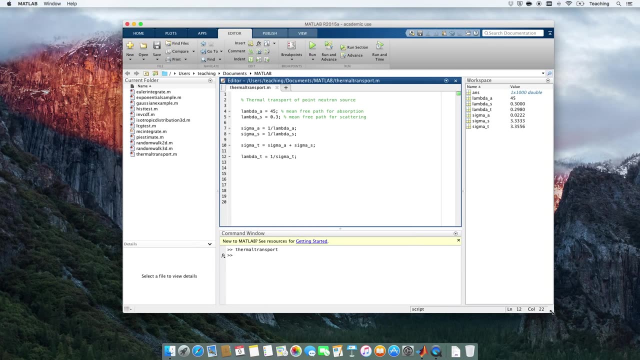 simply equal to one over Sigma t. notice that this total mean free path is going to be shorter than either of the either the separate mean free path for absorption and scattering. so just run that, see what it's doing and you can see on the right that it's calculating the absorption cross-section, the scattering. 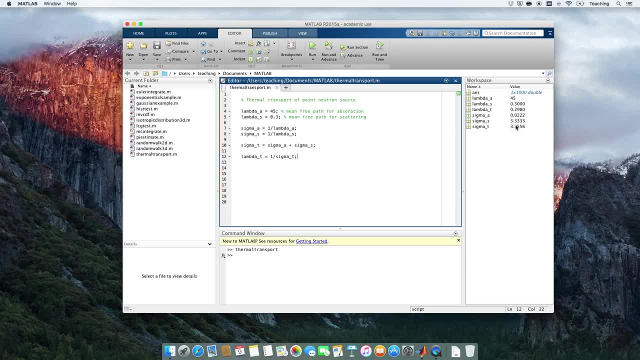 cross-section, the total cross-section, which is the sum of those two and the total mean free path, lambda t is equal to one over Sigma t, and we have a total mean free path of a bit less than 0.3 centimeters. now I guess I should do, should do clear all and close all at the 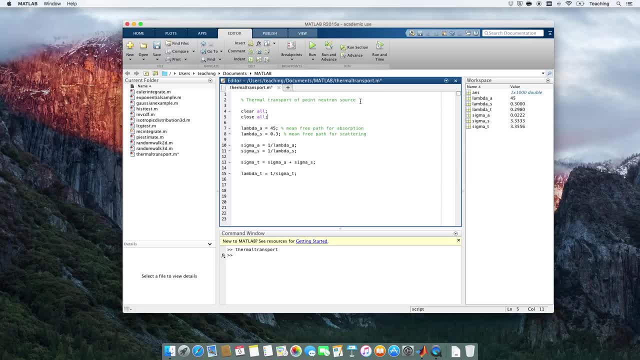 top, as we normally do, just to keep things cleaned up after ourselves as we go. now we're going to start neutrons from the origin, so let's look at one neutron by itself. to begin with, we want to follow its passage from its origin to where it ends up, so this is what's called the neutron history, and 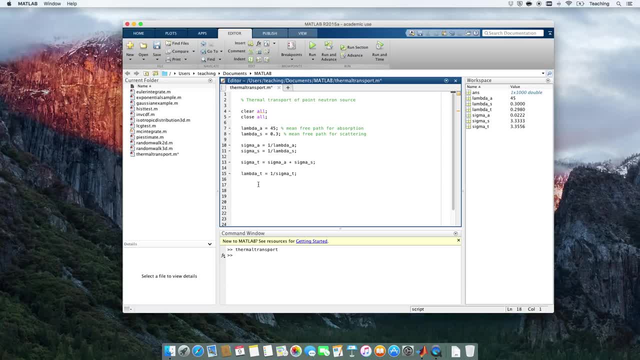 we are going to take a certain number of steps, but we don't know how many. so clearly we're going to need a while loop, so while- and I guess we'll need a flag for this neutron, so we'll say while not absorbed, and I guess we'll go to the. 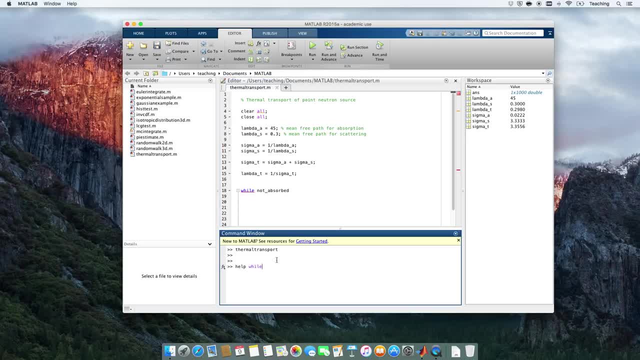 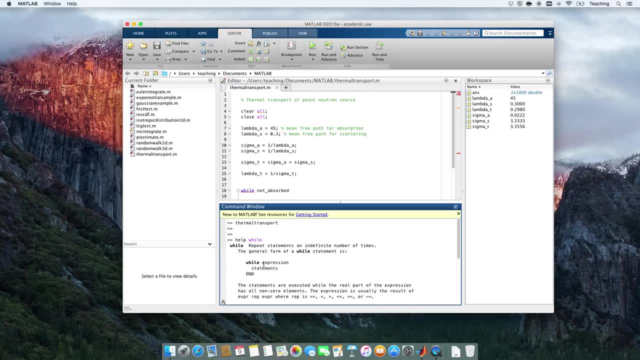 command line here and we'll just remind ourselves how a while loop works: while, and you can see that the while expression, while the real part of the expression, has all non-zero elements, while, it's true, so while not absorbed, and I guess we want to say while not absorbed equals one, okay, and I guess 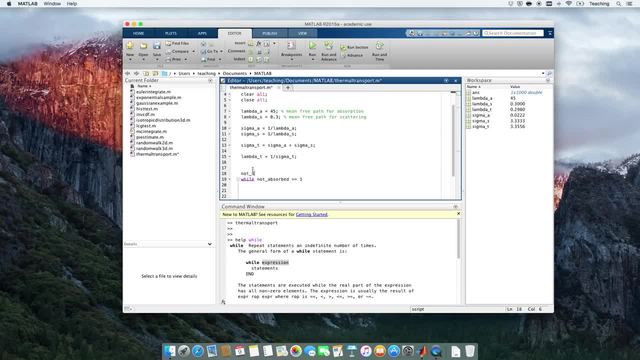 before we start that we need to set, we need to say straight away that initially, of course, it hasn't been absorbed yet, so we'll set: not absorbed equals zero. and since the neutrons are each starting from the origin, we'll say that the initial position X equals zero, Y equals zero. 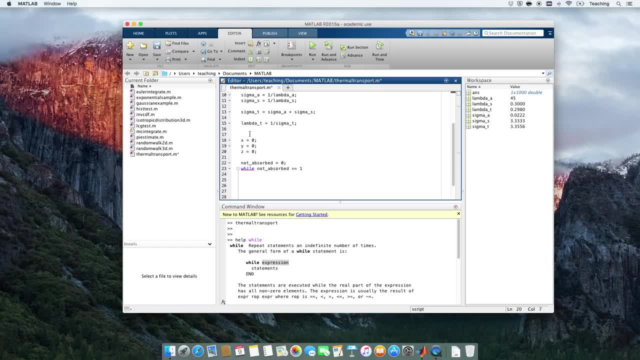 and Z equals zero. now, I'm not going to, I'm not going to follow the individual steps each neutron takes. I'm simply going to update its position until it gets absorbed, in this case. but in principle I could could put something like X, you know, X 1 here, and I could have X- I at the bottom here. but I'm not. 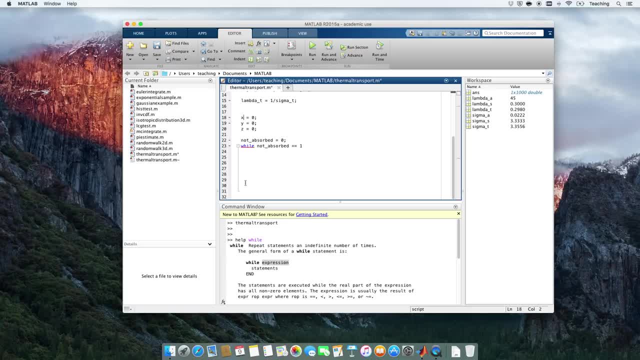 going to do that in this case. you see, I'm sure you can appreciate, you can do that. so I'll put an end at the end there. and for each step I'm going to calculate an isotropic step which is exponentially distributed. so for each particular step, 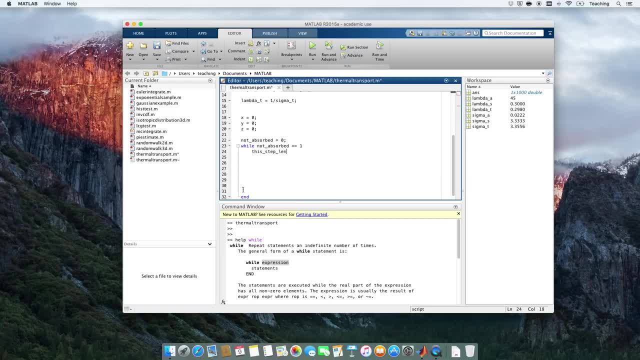 I'm going to call this this step length. I'm just going to call that s because it's a bit shorter, isn't it? s is equal to minus lambda T times. log of log of a random number. so that's my exponentially distributed step size and I want to. I 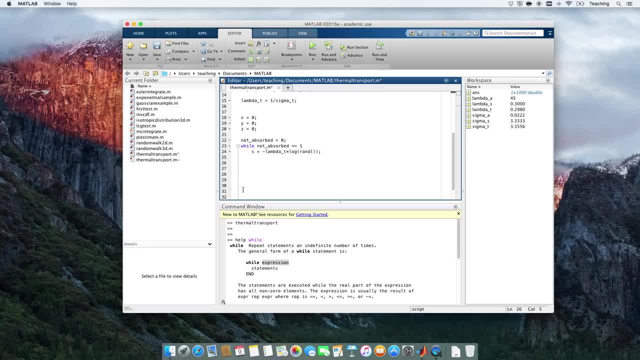 want to choose an arbitrary direction, so I need a theta and phi to go with that. so theta, the angle that the neutron happens to be going in, it's going to be the arc sine of minus 1 plus 2 times a random number. this will give us the correct. 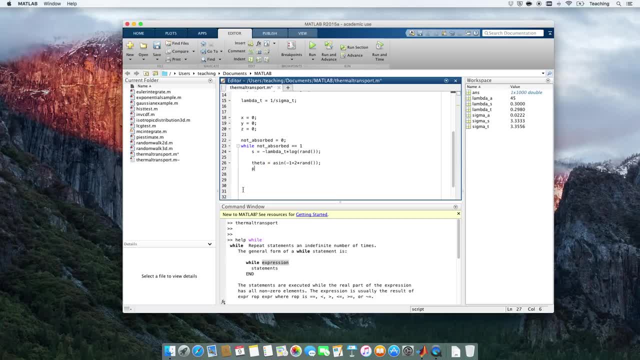 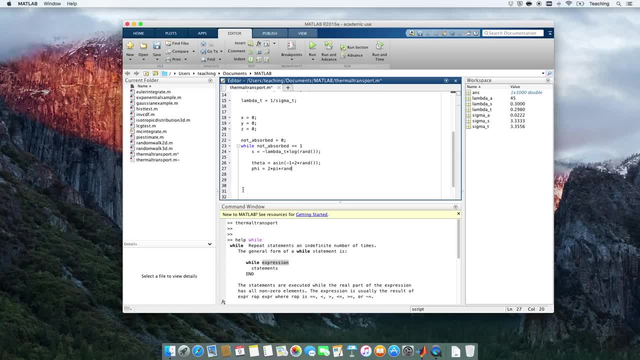 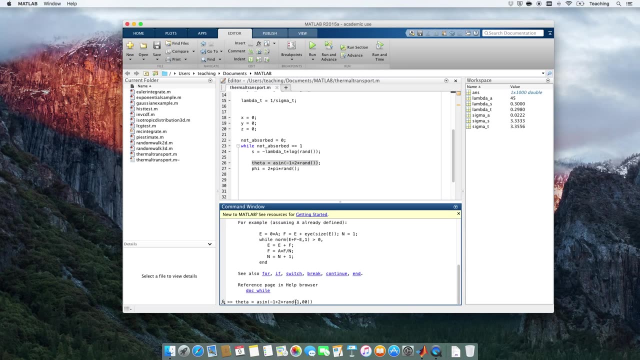 is equal to two times pi, times a random, and I'd like to let's just see what the theta values look like. so I'm just going to grab those here and I'm just going to make a table with a thousand of those random numbers, just remind myself. so I'm. 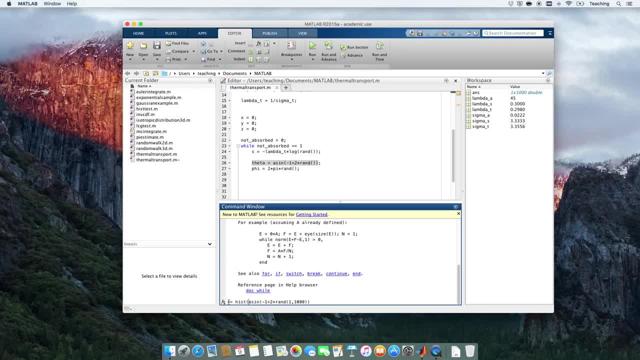 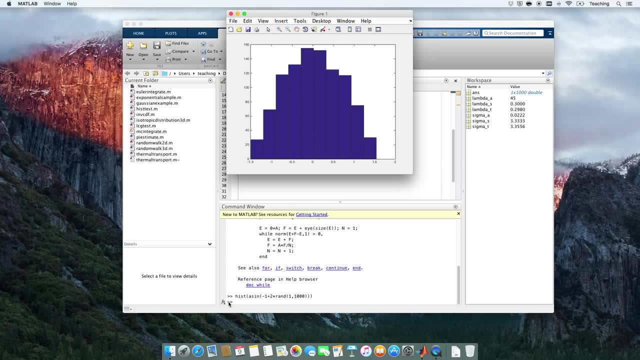 try creating a thousand of these numbers and I'm just going to histogram them to see what they look like, to see what values that we would get, And you can see they lie between minus pi and pi, So 0, where I have a larger density of those numbers occurs at the 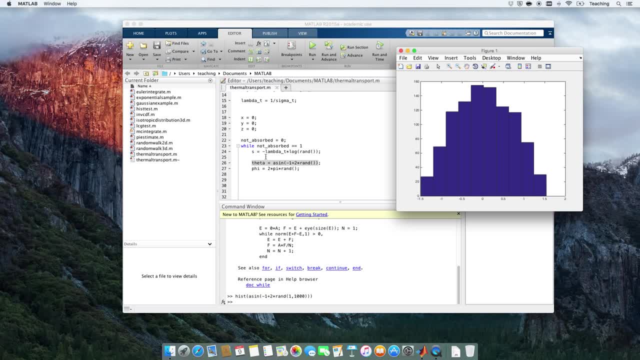 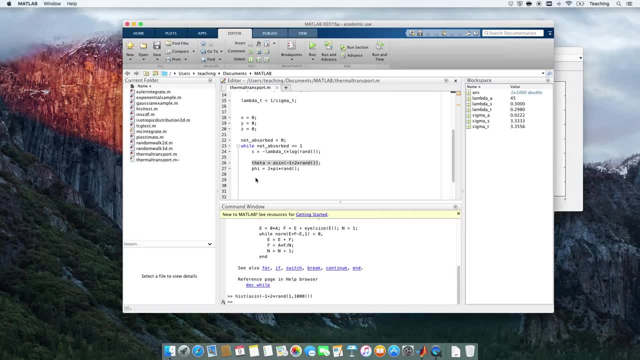 equator. So this tells me how to convert that theta value into the appropriate x, y and z value. So when theta equals 0, then z equals 0. So that means that z should be. in fact this is dz, because this is how the distance travelled is. equal goes as: 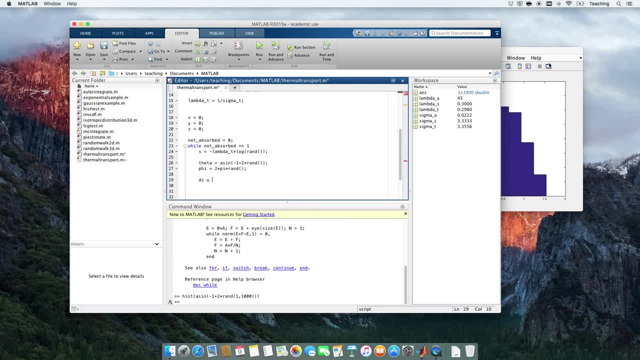 let's have a look back at this on the right here. so when it's equal to 0, z is 0, so it should go as sine of theta And of course the distance is s times sine theta. So therefore dx equals s times cos. 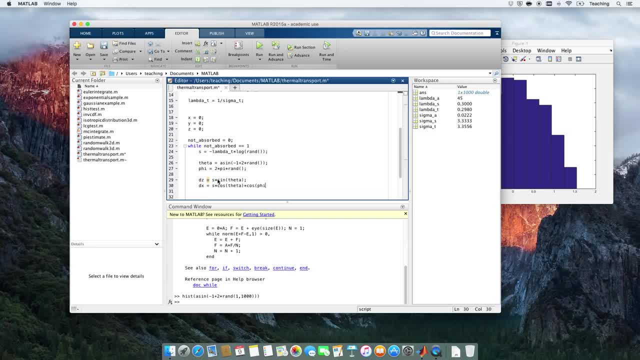 theta times cos phi, and dy is equal to s times cos theta times sine of phi. So what have I done here? I've created, I've created a distance for the neutron to travel and a random direction, and I've converted that into a step in x, y and z. So I'll just clean that up a little bit by. 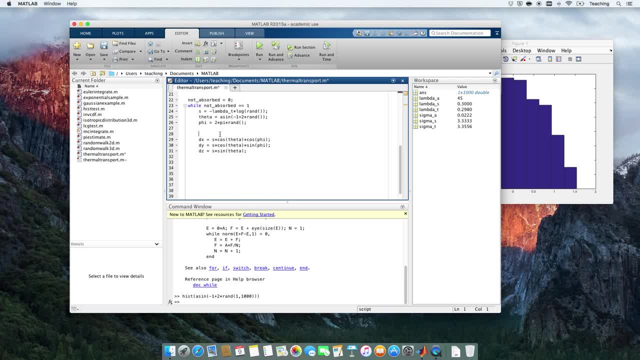 putting the z at the bottom, Just to make it a little bit less confusing. So all I have to do now to move the neutron to the end of the step is to say: x equals x plus dx, and so on: y equals y. 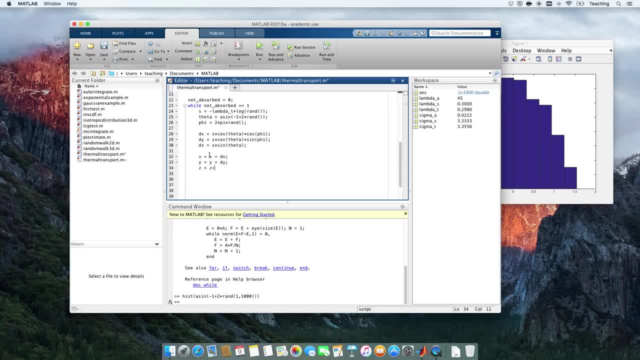 plus dy and z equals z plus dz. Now the idea of a mean free path is, of course, that at the end of that distance something has happened. So I have to apply a physical process at the end of this step. So at the end of the step, I ask myself a question. 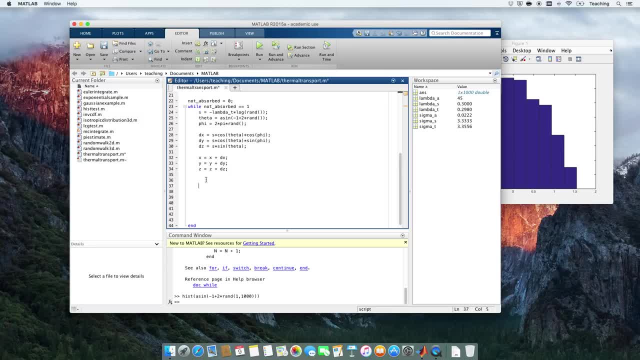 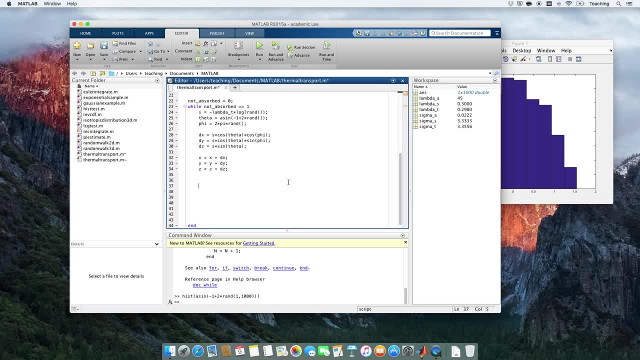 Has the neutron been absorbed Well? how do I know the probability that that neutron has been absorbed Well? how do I know the probability that that neutron has been absorbed? If the mean free path, if it was only scattering that was occurring, then it would have a short mean free path and at the end of each step, 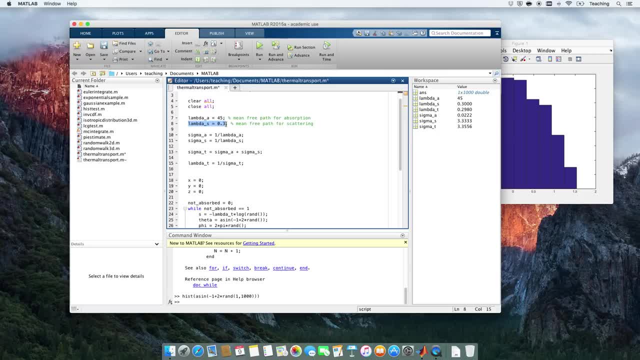 a particle would scatter and to continue to scatter and to move, and we're going to assume that at the end of each step the neutron would operate improperly. the resulting direction is also random. so because the neutron is thermal, and we're going to assume the water, 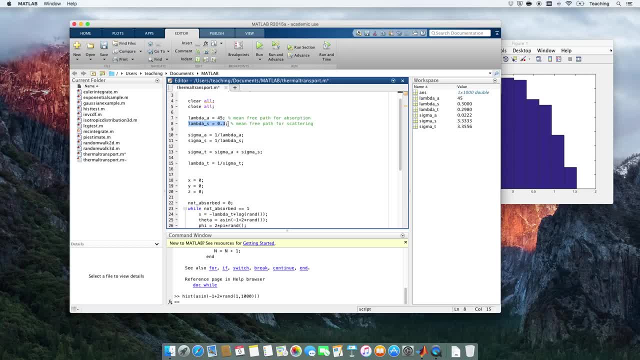 which it's travelling in is at the same temperature. these two things are in equilibrium then. loosely speaking, the direction the resulting neutron comes out at after it's been scattered is random in direction. so all I have to do here is I simply have to choose the relative probabilities. 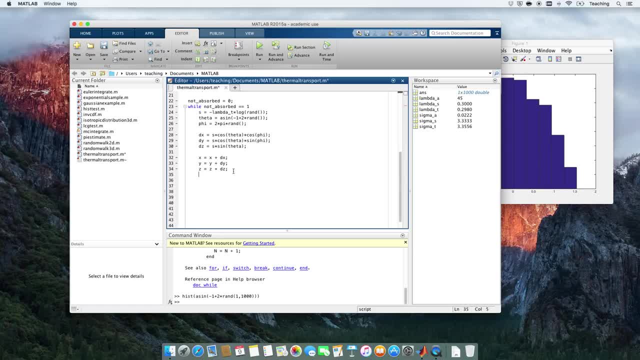 of absorption and scattering. well, that's quite easy to work out. what I have to do is I roll a random number. so I say, if a random number is less than sigma A divided by sigma total, we'll have to just check. this is the right way round. 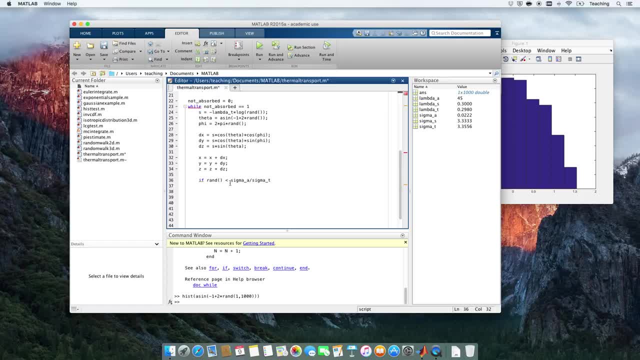 so what are we trying to say? if this is a number between 0 and 1 and this number on the right is, what proportion of the total macroscopic cross section is the absorption? so what we're saying is: if the particle is, if the particle is. 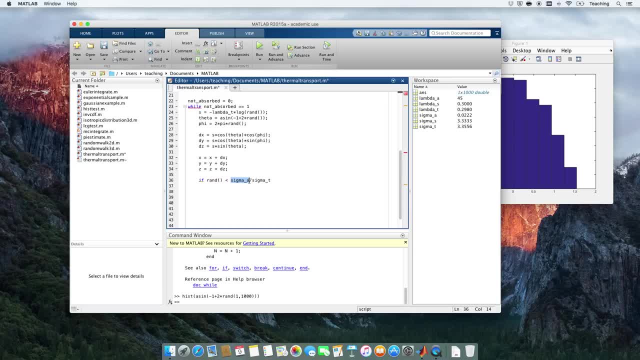 if we roll the dice and the particle is absorbed, then we wish to stop this calculation. so if this random number is less than this ratio, then we're going to say that it's absorbed. so what we'll do is we say: say not, that's what we should say. 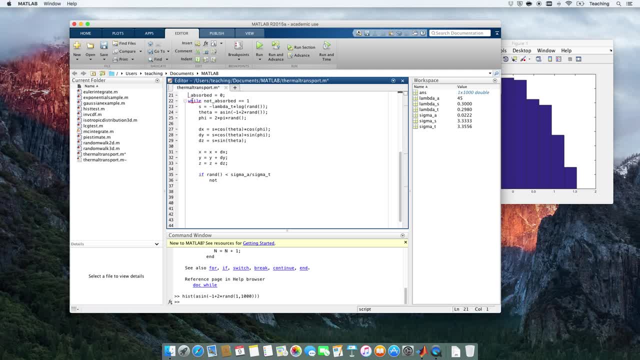 is absorbed at the top. here, just to make it a little clearer, we'll call this: is absorbed at the top if is absorbed equals 0, and then, while is absorbed equals 0, just rewrite our meaning of what we're doing here and we'll say: is absorbed. 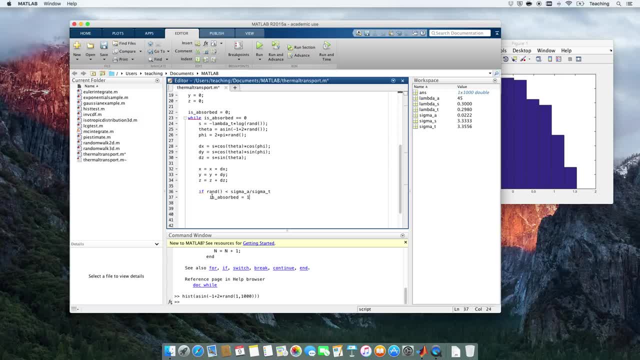 equals 1 at the bottom. I'll just remind myself if I need an end statement at the end of my statement, which I do in this case. so I'll say end and I think that's it. so what have we done? we are taking steps in a random direction. 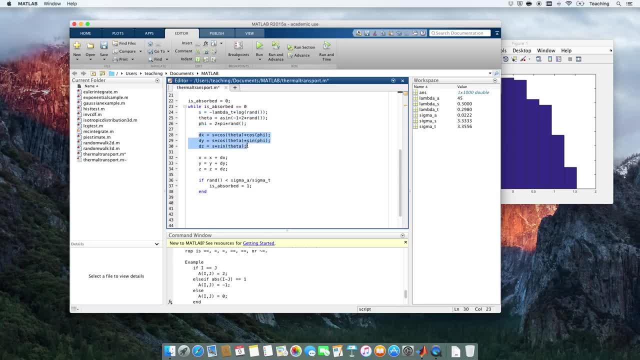 which is what this is doing. we're calculating dx, dy and dz values for each of those steps and at the end of the step, we simply decide whether the particle has been absorbed or not, and if it's been absorbed, I set a flag and I stop doing the tracking. 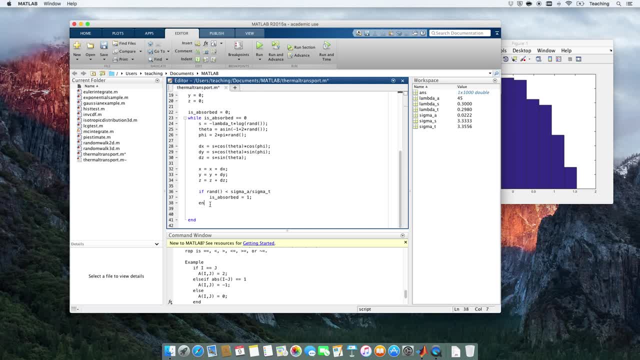 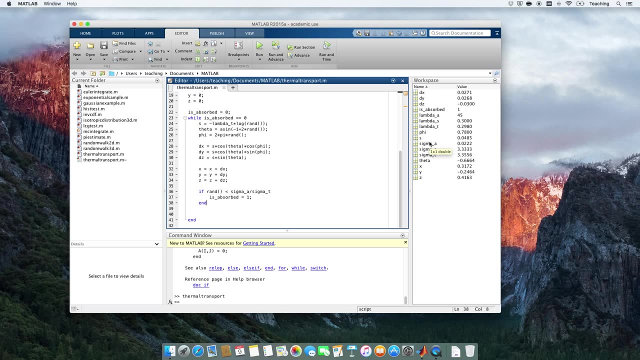 and, and and. if it hasn't been absorbed, then this while loop will continue and I will continue to update the position of the neutron. so let's see if this actually works. let's run it. this is running for one neutron and you can see that when we run it. 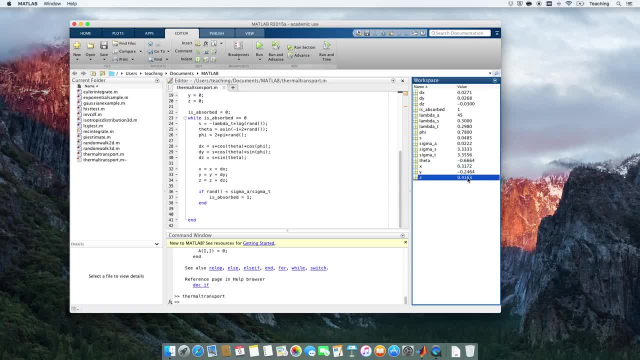 you can see that it is actually producing some outputs, producing some x, y and z values which are different from 0, so we think that something is happening. let's have a look how many, how many steps that we need to do here, how many steps that particle took. 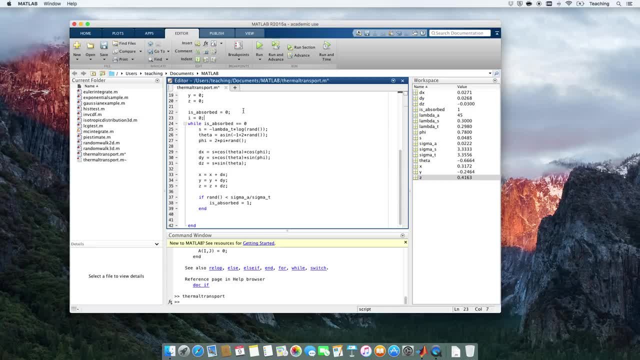 so I'll call this: i equals 0, and then for each time I make a step I'll do i equals i plus 1, and I'm just going to keep track of that variable to see what happens. so let's have a look when I run it. 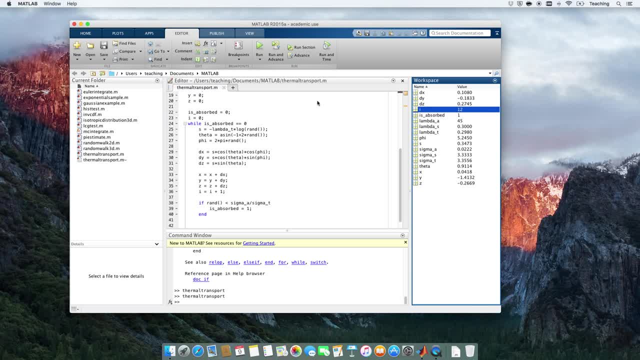 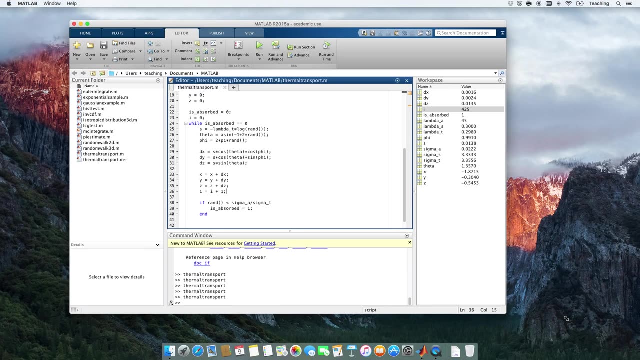 you'll see that a variable i, so you can see I've taken 12 steps. let's run it one more time, and this time it took 14 steps. run this again: oh, 223 steps, a very large number, and 425 steps. so perhaps we can use that i value as a check. 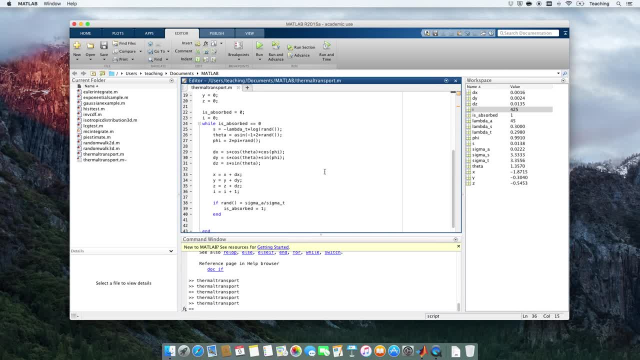 to see if things are working as they should do. I mean, how many steps should we be taking? well, if we look at the ratio of the cross sections, which is 3.3 divided by 0.02, that's, on average, how many steps we're taking. 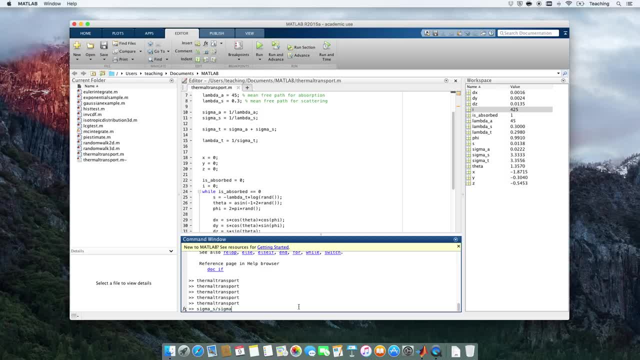 it's the ratio between those two numbers. so sigma s divided by sigma a is about 150. so we should be taking of the order of 150 steps. so we're going to take 3.3 divided by 0.02, so 150 scatters occur before an absorption. 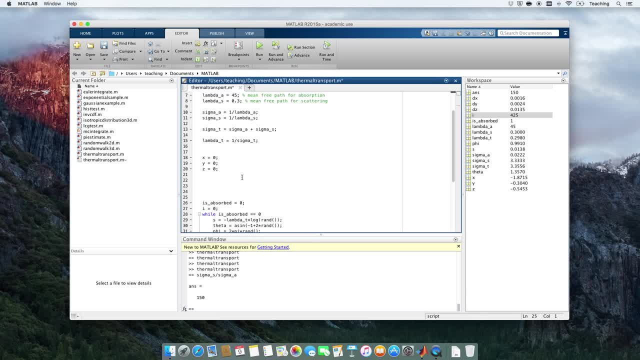 so what we could do is we could put a for loop around all of this. in fact, we should put the for loop up here, shouldn't we? so let's make a for loop. so we'll say: n particles equals 1000, so we're going to count 1000 particles. 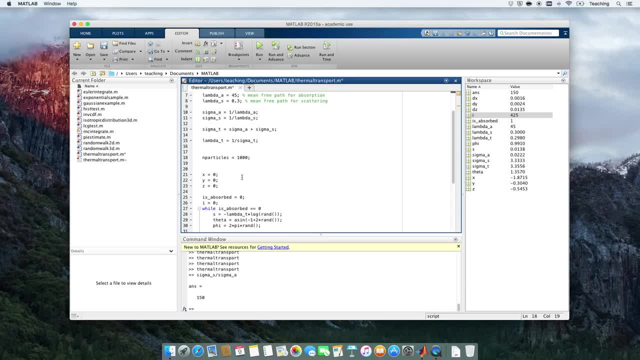 we could also call this a number of histories, because of course, these are not real neutrons. we're modelling, we're using, we're looking at one neutron at a time and we're calculating the statistical properties of neutrons and neutrons with many of those individual histories. 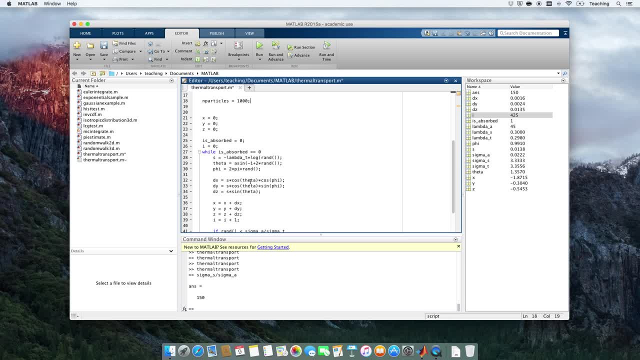 in order to estimate what's happening for a typical neutron. so for each one of those we need a for loop, for j equals 1 to n particles, and each time I do that. so let's put an n statement at the end down here, and I should really indent this code now. 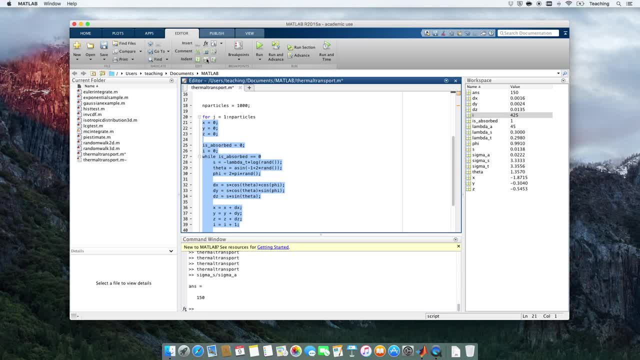 so each time I run a history, there's the indent, there's the indent, there's the indent. so let's, what am I doing? I'm doing 1000 runs and each time I do a run I start a neutron at the origin. I say it's not been absorbed yet. 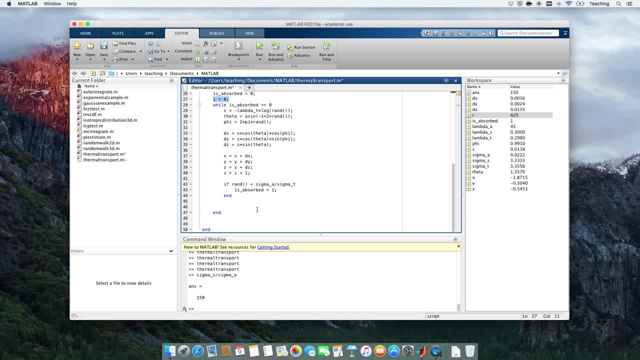 I count how many steps it's taken and also where it ends up, and the first thing I can do is I can count up how many steps. let me make this clearer. I'll call this historyLength beside here. I'll just call this historyLength. think something like that. history length J, so J will run from 1 to n particles. 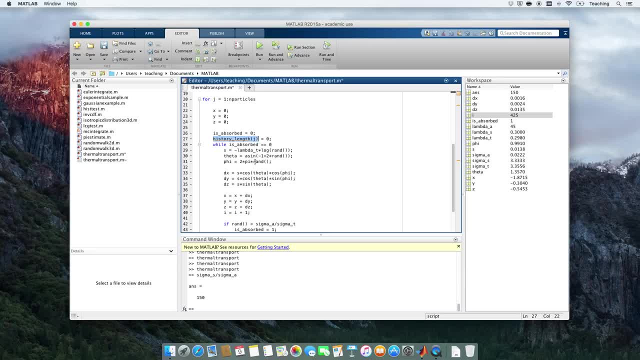 and then, every time a particle is scattered, I add 1 to that value. there we go, and what I could do now for each particle, I'd say X J equals 0. okay, so of course I should really initialize these arrays at the beginning, but this will. 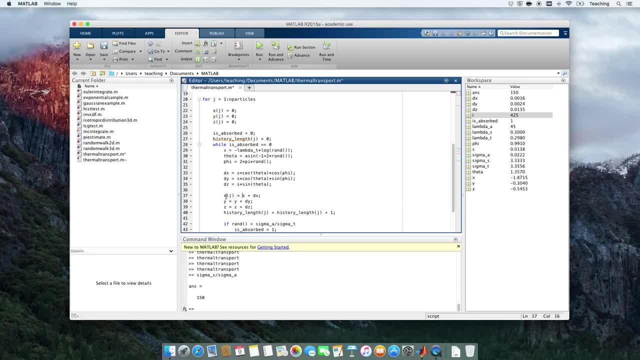 still work fine, and I'll say X, J. so what I'm doing is each particle, I'm updating its position as it moves through the water and at the end I have the position of those particles. so I think that should work. so that's what I'll do, is I'll run that and see if it works. 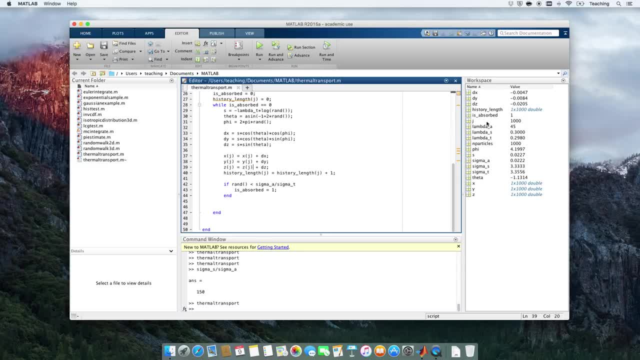 yeah, there we go, and I've created a thousand values of J, thousand values of X and a thousand 1,000 values of history length. So what is the mean or average in mathematics? I think it's mean. Yes, it's the mean. So the mean value of the history length, I press tab. 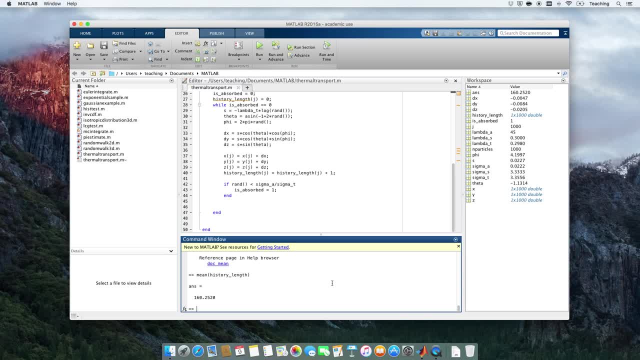 is 160.. So that's not too bad. It's not far off. Let's see if I run it again and see if it gives me roughly the right value. I'll run it one more time. So the mean value of 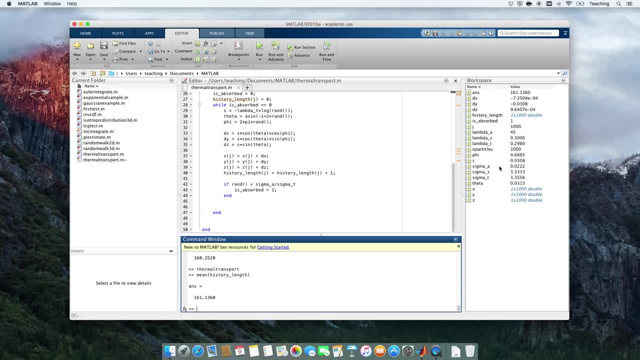 the history length is 160.. That's a little bit off. Did I calculate? Did I? Maybe I haven't put all the accuracy that I need in there? If I divide 45 by 0.3,, 45 divided by 0.3 is: 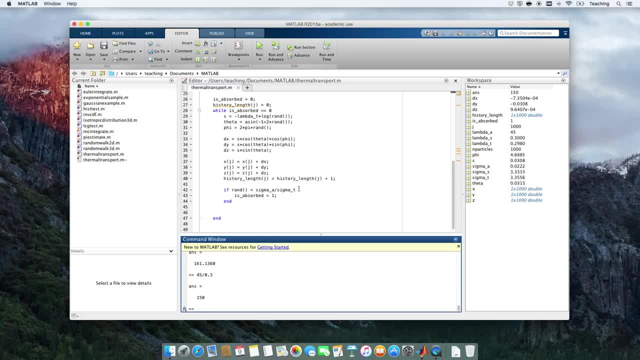 150.. So for somewhere there's a slight error here in how many seconds. So I'm going to see how many steps I'm taking. You can see I'm taking on average 10 steps fewer than I might imagine I should be taking. I might have to look back at that at a later time. 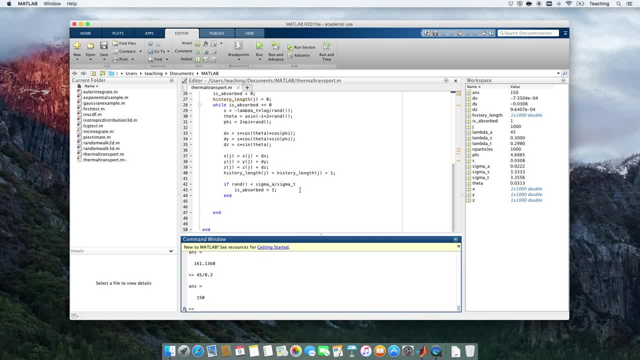 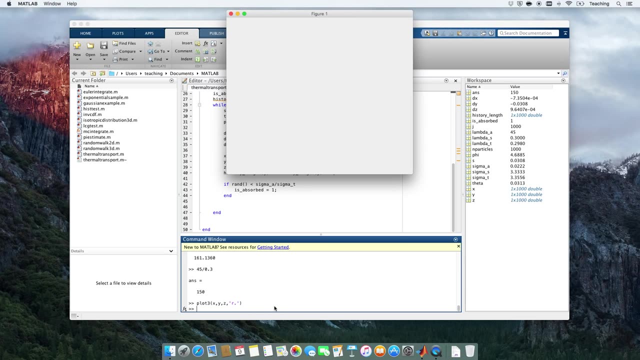 But I think more or less it's working correctly. So anyway, let's look at what the particles look like. So let's look at the final positions of the particles. I'll do a plot 3 of the x, y and z's And I'm going to do red dots. Let's have a look at what that looks like. 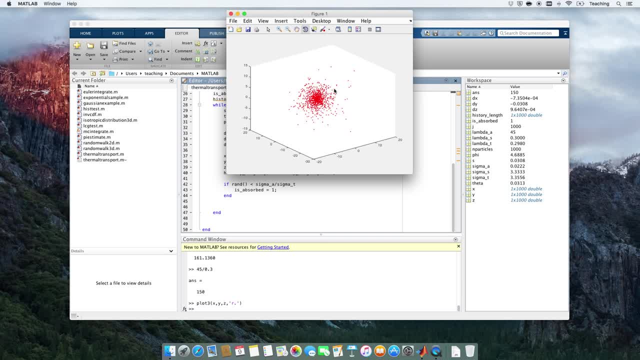 And that's where all the neutrons ended up. So some of them go quite a long way and some of them don't go so far, And perhaps that looks about right. So we'll need to have some kind of sensible checks to see whether 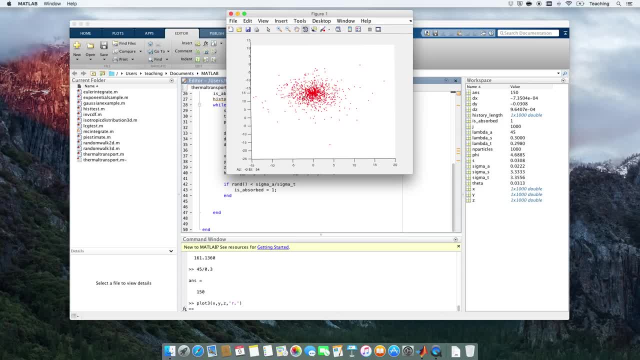 that really is true or not, But you can see that if we think that the mean free path for absorption is around 45 centimetres, but remembering that when the particles scatter they can be bouncing backwards and forwards, then perhaps a typical distance travelled of 5 centimetres. 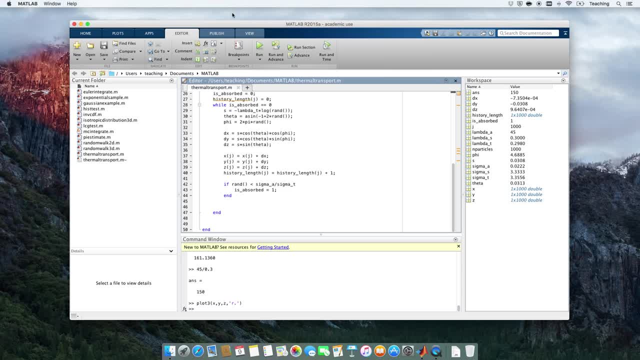 is not so bad. So let's find out what the typical distance travelled is. Well, how are we going to do that? We can work out for each value. So this is here. we are following each neutron history. We can calculate the distance travelled as rj. 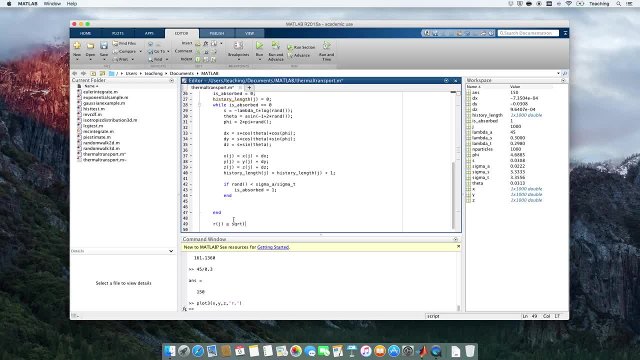 is equal to the square root of xj squared. And then we'll just do plus, plus, and we'll do x, y and z. There we go, And this will obviously be a positive number. So at the very end of the 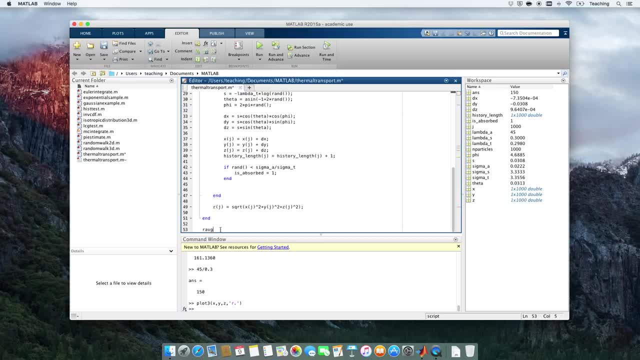 calculation I can calculate r average is equal to mean of rj, So this is the rms distance travelled, And so if I display that as well r average, then we get a typical distance travelled of 7.6 centimetres. 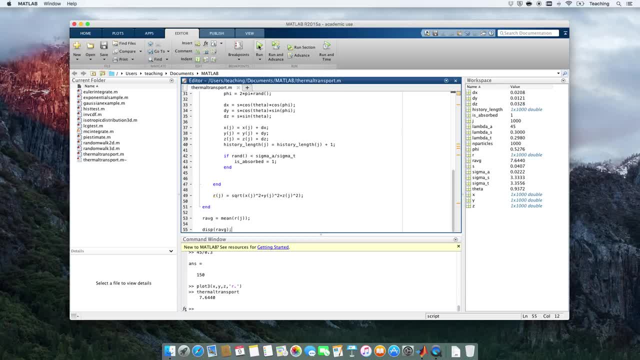 So an interesting question we can ask about all of this is how many particles get to a particular distance. So rather than calculating the mean distance travelled, we can count how many particles per particle generated are getting a distance. say, well, you can. 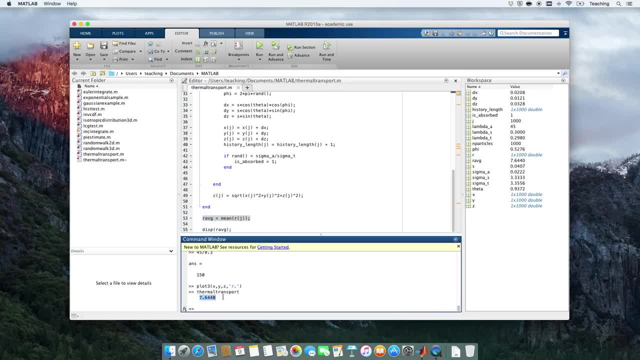 see here that the typical distance travelled is about 7.6 centimetres. Let's count up how many neutrons are transported to 10 centimetres, So this is called a tally. So we've calculated the mean distance travelled. but now let's 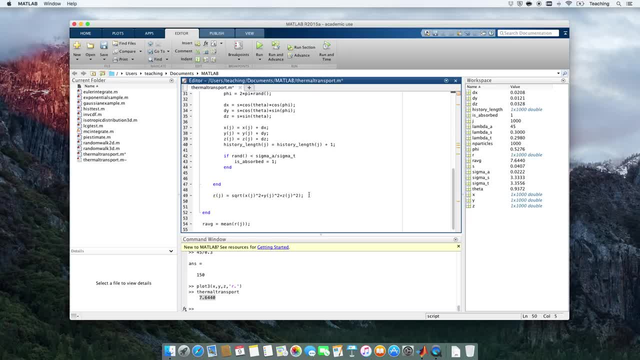 say, we'll calculate two tallies. One is we'll say t out and t in, So by which I mean this is the number of particles generated. So this is the number of particles greater than 10 centimetres, and this one is the. 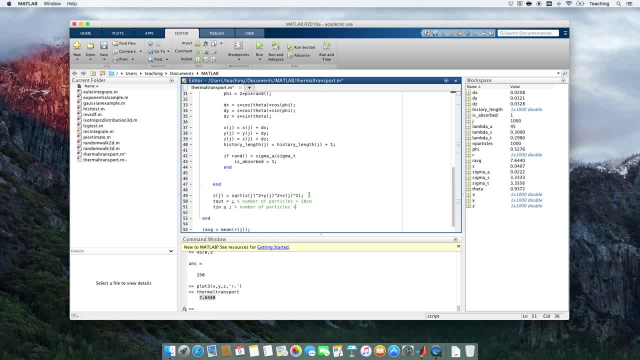 number of particles that didn't make it 10 centimetres. So in order to do this tally, we need to. when we do our for loop here, we need to initialise before we start actually. so it has to be outside this for loop. we need to initialise. 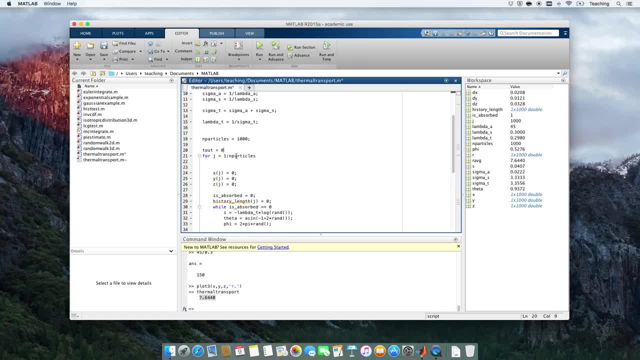 we need to say that t out equals 0 and t in equals 0. So what we have to do is we have another, we have an if statement that says: if rj is greater than 10, put an end here and just tab in here and say else. 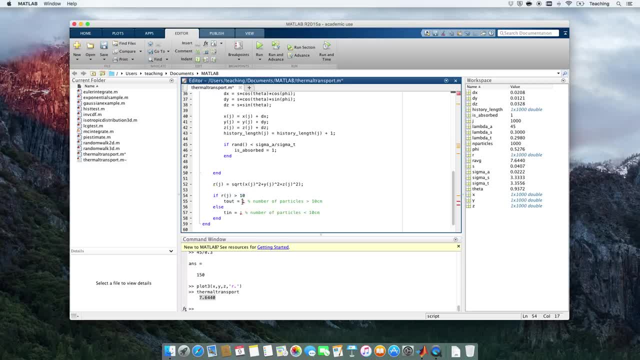 So if the particle travels more than 10 centimetres, then we add 1 to this tally, t out plus 1, else Otherwise we add 1 to the other tally And see if that works. we'll just run it to make sure it's working. 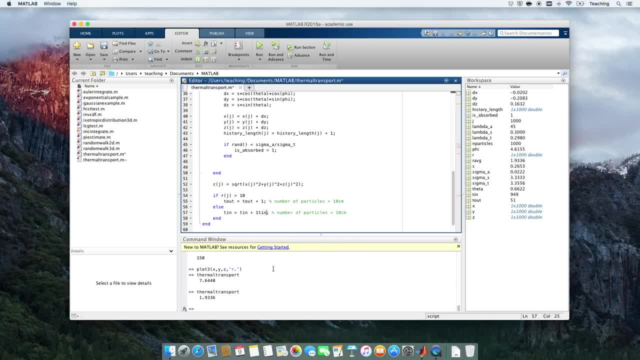 Now let's check that everything is as it should be: t in plus oops. let's go to the bottom here. So t in plus t out should be equal to 1000, which it is. Let's just check. that's always the case. 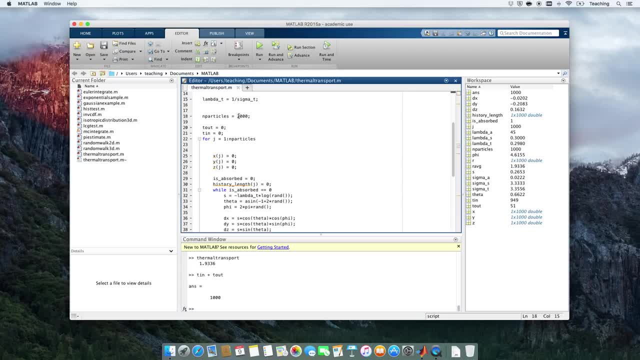 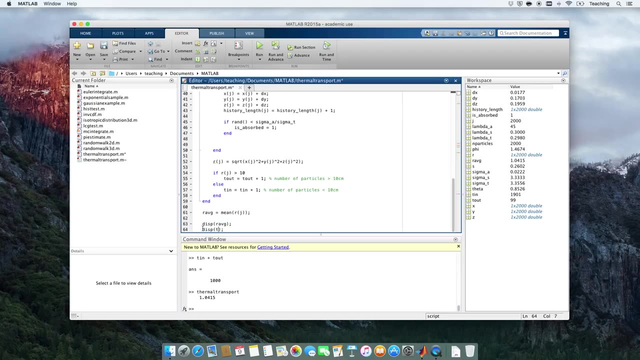 Let's do it for a large number of particles, say 2000.. And run this again, And in fact we probably should display t in plus t out. In fact I just noticed something. actually, That first run we did seemed to be anomalous. 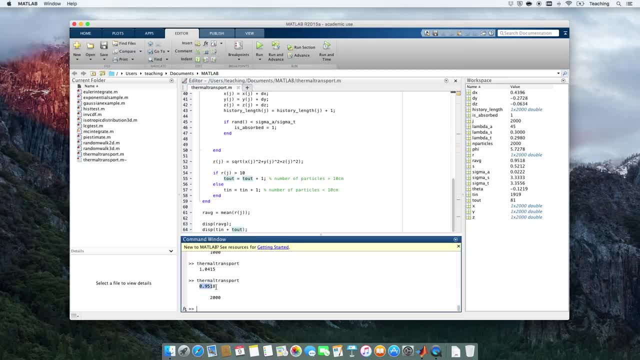 If we run it for a large number of particles, the typical distance travelled is 0.95 centimetres, which is a lot smaller than we had initially. Let's see if that's always the same. Let's just do a test. 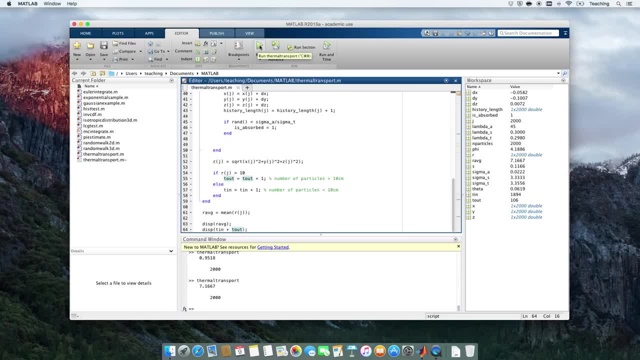 So we can test to see that everything is behaving itself. We might have to debug now. So we run it again. We get 4 centimetres, 7 centimetres, 9 centimetres, 1 centimetre, 1 centimetre. 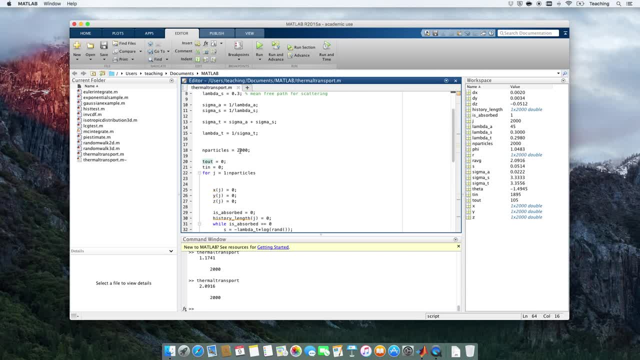 Does that behave itself without having to properly debug? Let's see if it behaves itself. if I have a smaller number of particles- 6,, 3, 2. So there's quite a large fluctuation in the mean distance travelled. Have we done everything correctly? 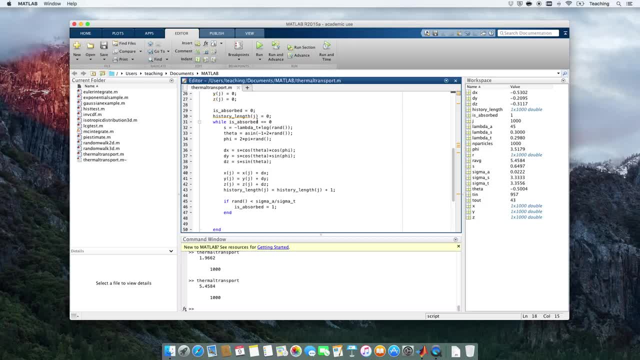 Let's have a look down here. So each time we make a step, we always make at least one step. So the minimum value of history length should be equal to 1.. So let's see what the minimum of history length is. 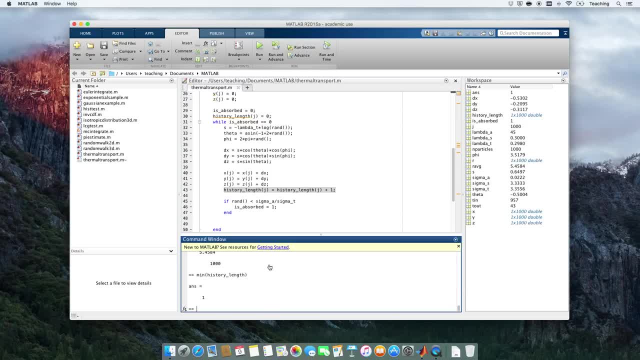 The minimum value of history length is 1. And of course that will on average be true. It won't always be true. Sometimes it might be larger. All this seems to be OK. I think We're using the correct mean free path here. 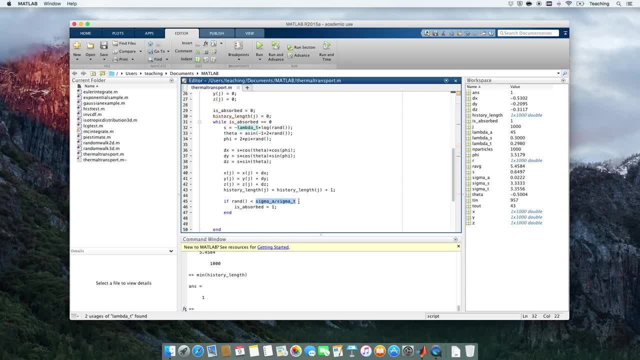 And we are correctly looking at absorption versus the total cross-section here. And let's just check- we've done the calculations right up here- The absorption cross-section is 40.. So absorption mean free path is 45 centimetres. The scattering mean free path is 0.3.. 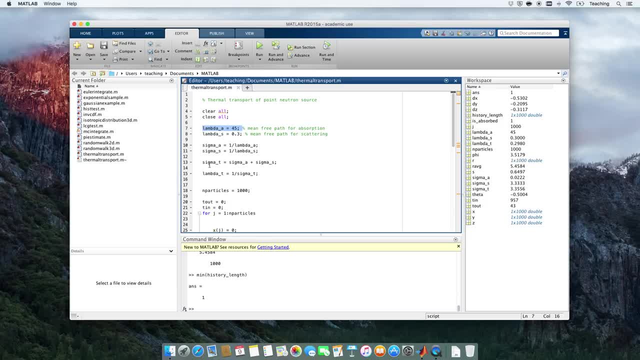 We correctly calculate the macroscopic cross-sections. We add them together. Calculate the total mean free path, Have we? Yes, we're using the total mean free path here, So I think everything is right. I'm still a bit puzzled about the typical number of steps. 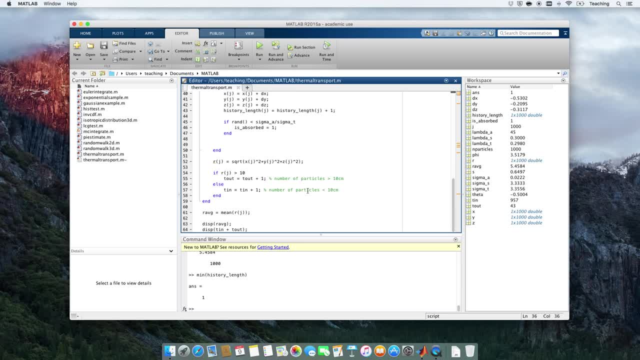 I might have missed something there. I might have to check that another time. Now let's look at these tallies. So what was the tally in this case? Let's have a look. T in was 957. And T out is. 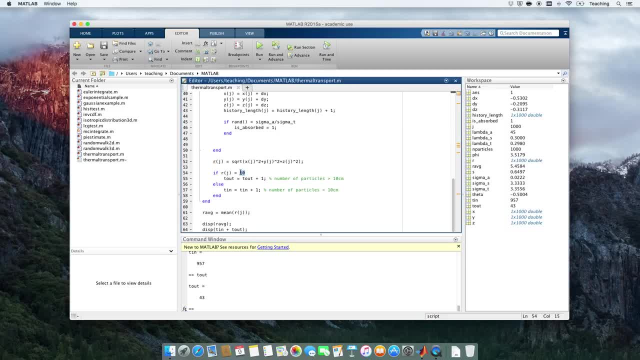 About 43. So if we were to reduce this- Let's count the number of particles that make it to 5 centimetres- We should have a larger value of T out. So if we look on the right here, So when we count how many particles make it to 5 centimetres, 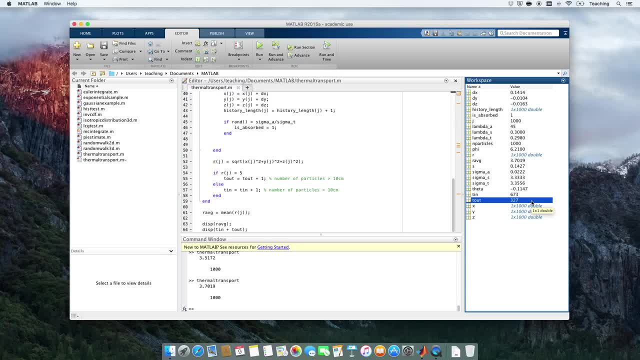 Then about 300 of them are getting to that distance. So what is that telling? So that's telling us that if I have a neutron source of a given strength And I stand, I stand 5 centimetres away from it. 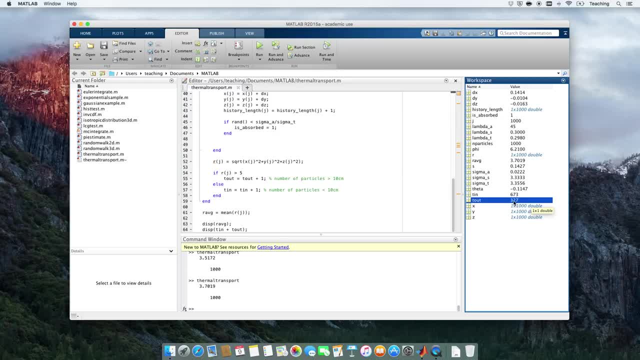 Then or I put a receiver 5 centimetres Or a detector 5 centimetres away from it, Then around about 300 particles get to that distance. So of course, to work out the flux I need to calculate the area over which I'm detecting. 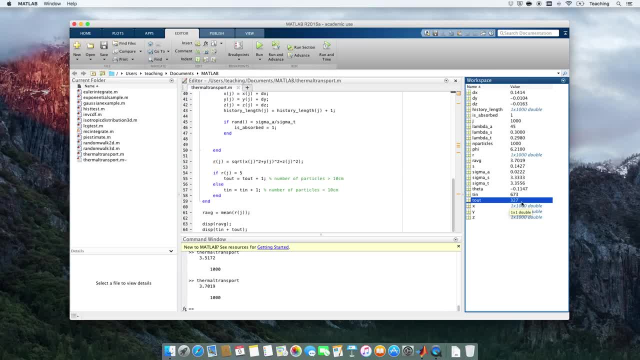 And Or receiving that radiation, And multiply it by the, So multiply 327 by the fraction of the total surface area At 5 centimetres, So I can now work out the neutron flux Going through a particular area at that distance. 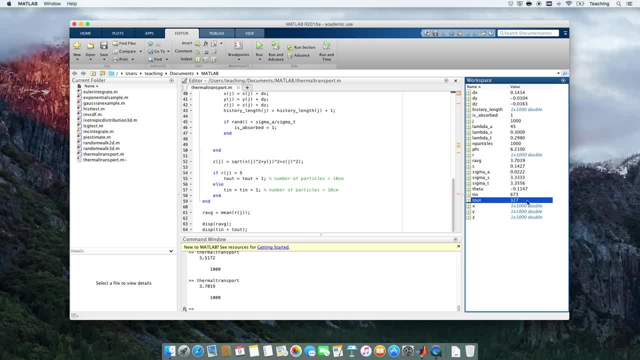 So I'll leave that as an exercise for you to do Now. what's interesting here is: To what accuracy do I know, To what precision do I know T in and T out? Well, a rule of thumb Is that, loosely speaking, 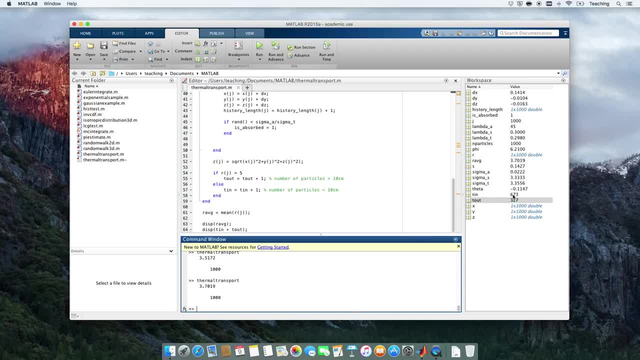 The standard deviation of T in and T out. T in and T out Is the square root of those two numbers. Now when I only have two possible outcomes Of them, tallying up Either inside or outside, Then actually that rule of thumb is not correct. 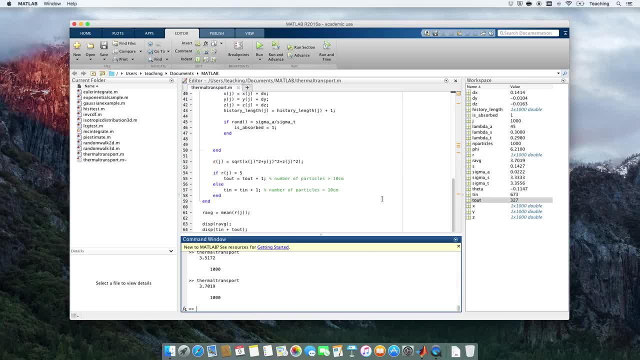 Let's see if we can run this several times And we can calculate the variation of T in. So let's look at what we think the error bar of T in is. The T error bar we think of on T in Is about 26.. 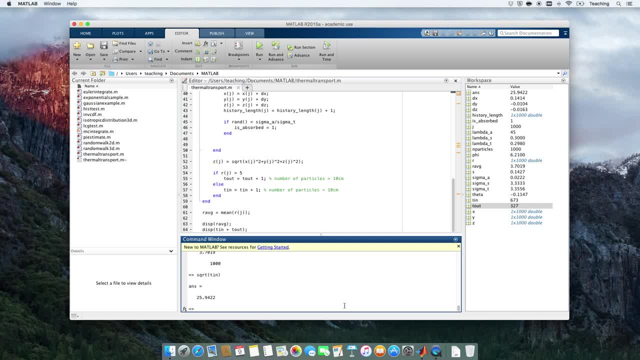 So our quoted answer could be something like 673 plus or minus 26.. Let's actually calculate what it is By doing this calculation several times. So what I'm going to do Is I'm going to put just another for loop around here. 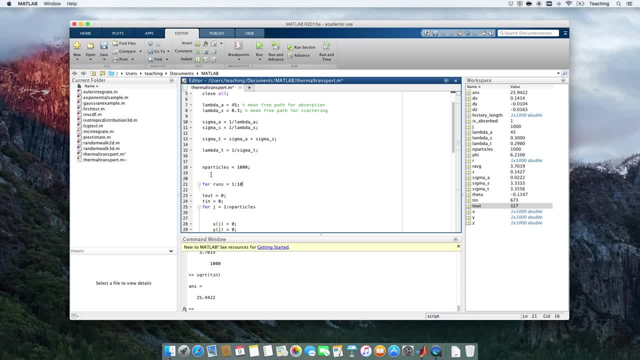 And I call this for runs equals 1 to 10.. And I'm going to go down to the bottom And I'm going to do: Let's go right down to the bottom here. Another end statement in here. So this code: 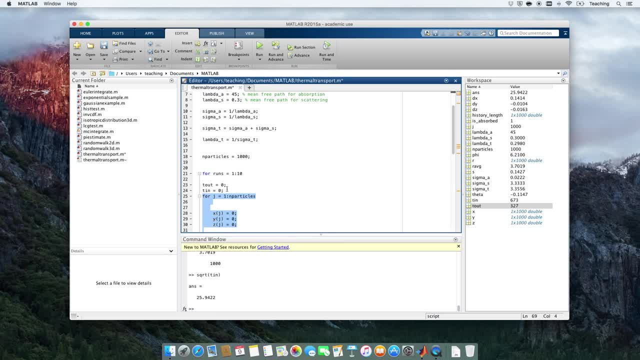 You can see, I'm gradually building up A larger and larger bit of code, So I'm going to indent this again. So what am I doing? I'm running the whole calculation of 1000 neutrons. I'm doing the whole calculation of 1000 neutrons. 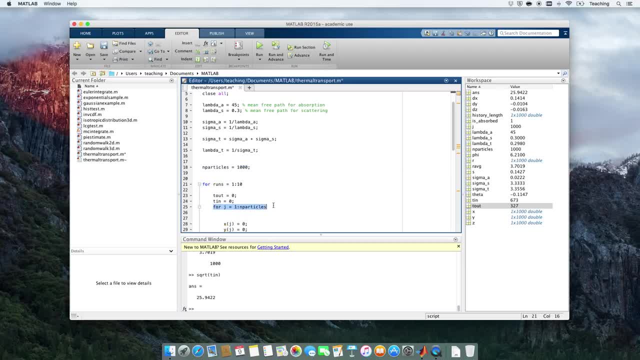 And I'm going to do it 10 times. So 10 times I'm doing the calculation of 1000 particles here. So each time I do that, I want to calculate. Let's look at T in, Because that's what I started looking at. 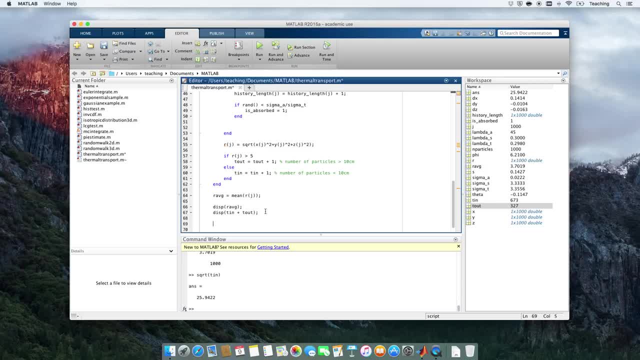 I'm going to count how many particles stay within 5 centimetres. So I'm going to say tally in is runs. So that's the number I need. That's the run number I've got, Which is 1 to 10.. 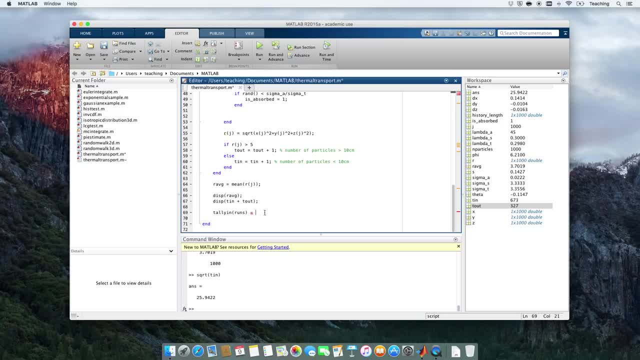 I'm going to go to the bottom here. Tally in runs is equal to T in. Let's just do it, Because we can, for particles that go outside, And tally out is equal to T out. So I'm doing the calculation 10 times now. 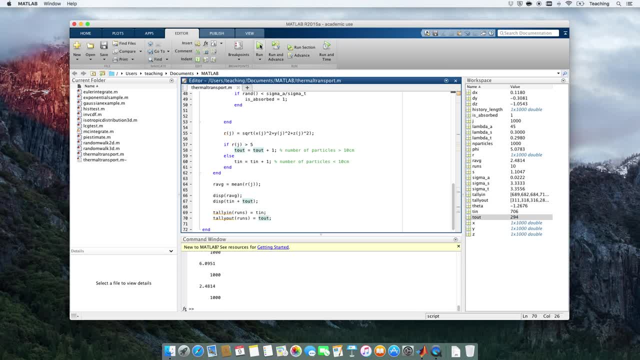 It's going to take a little bit longer. There we go. So you can see that tally in is a list of all the individual answers from the 10 runs. So if I calculate the standard deviation, Let's have a look. 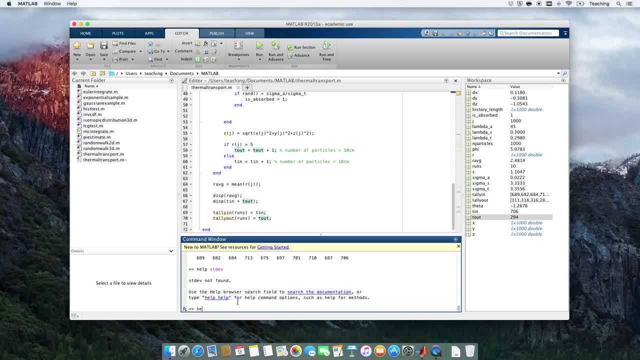 Is it help? stdev, I think it is in this case. Oh, std isn't? it Isn't that flat? So std is the standard deviation. So if I calculate the standard deviation of tally in, Then the value is actually 12.. 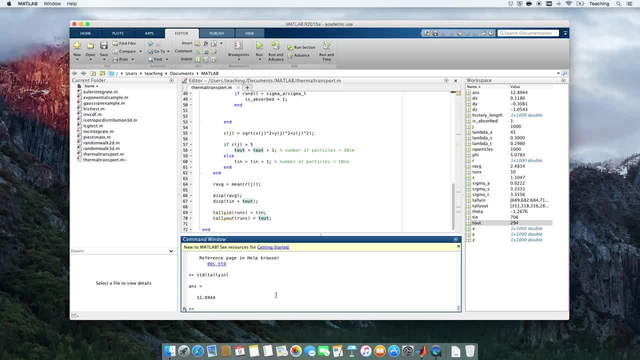 It's a little bit smaller than what we did. If we take the mean value, The mean value of tally in, And that's 694.. So the square root of that Mean tally in There we are. So you can see that the mean value. 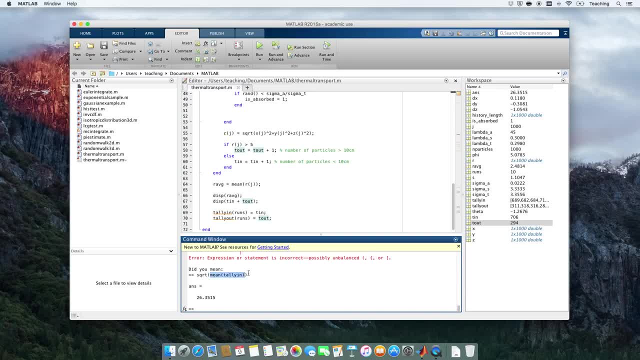 Yep, The mean value of the number of particles that didn't make it past 5 centimetres Is around 694.. About 694 particles in 1000 don't make it past 5 centimetres, And our rule of thumb calculation 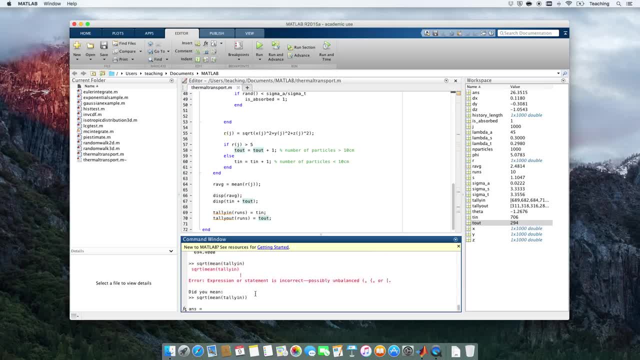 That the error is plus or minus 26. Is actually too big And the true error is, Looking at the standard deviation Is more like about 13. It's a lot smaller And that's because that rule of thumb doesn't work. 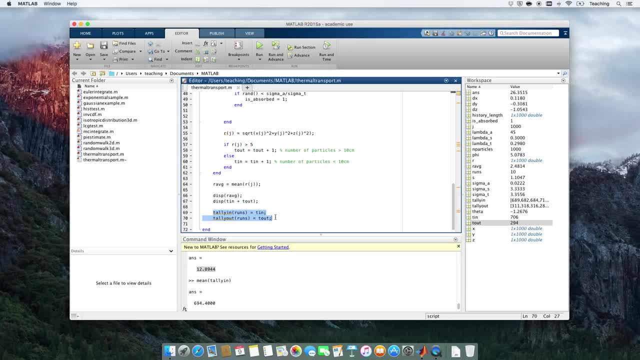 When I have a very small number of tallies, Because actually it's binomially distributed Rather than normally distributed. Let's look at the values. Let's look at the mean value of tally out. So about 300 out of every 1000 neutrons. 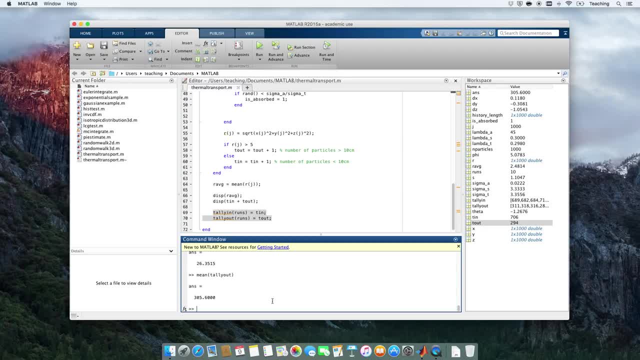 Make it past that 5 centimetre radius And the standard deviation of those values Is about. Tally out Is around 13. again, Did I do that? 13 before It works? It's about the same, Okay. 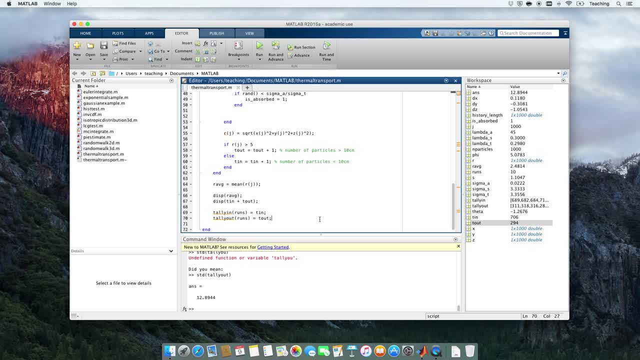 So that's it. So that's a neutron transport code. Now, what have we missed in our complete description? Well, obviously, I've assumed that the particles, for simplicity, All start from the origin. They needn't start from the origin. 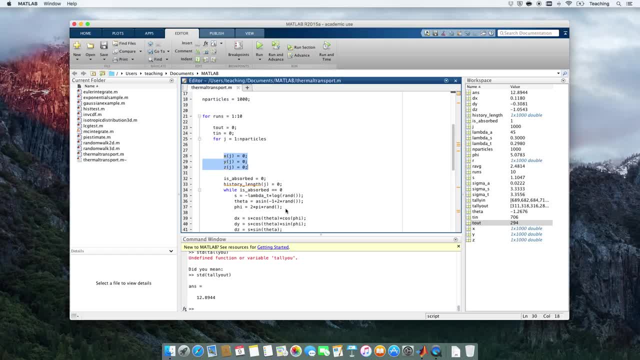 I've also assumed that everything is isotropic. So the initial direction is isotropic And all subsequent scatters are isotropic. So in a real radiation transport code, Neither of these things are likely to be true, But I've just assumed they are for simplicity. 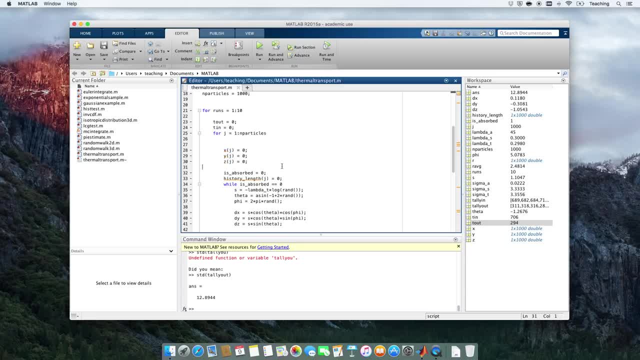 Now the other thing I've assumed Is that there's no change in the neutron As it travels. So if we look up here, These mean free paths Are considered to be constant. In this model that I'm applying, They don't change. 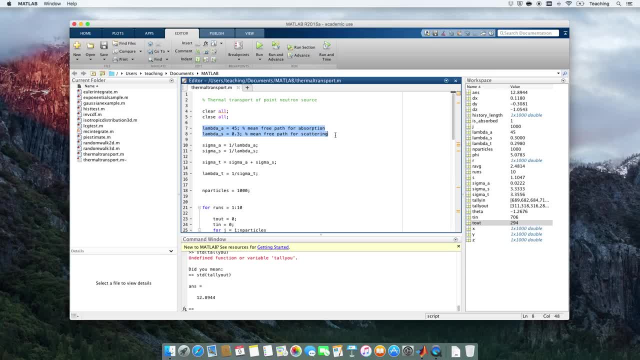 And so the neutron can't change energy And therefore doesn't see a different mean free path Or, equivalently scattered cross section. And of course, the other thing Which is true in many cases in reality, Is that the neutron can't do anything. 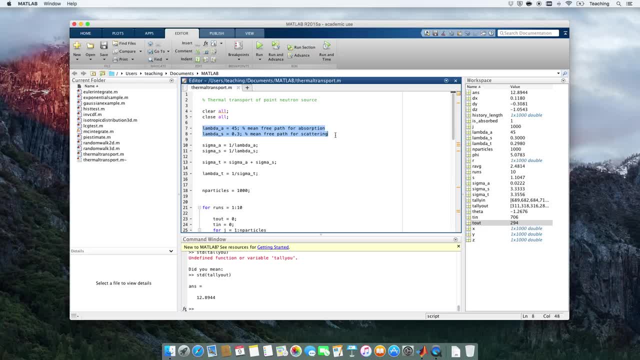 Other than being absorbed or scattered, There are no other physical processes. There could be other things it might do, Such as it might induce another neutron to appear. It might turn into other particles. So more sophisticated codes Will take account of all of these things. 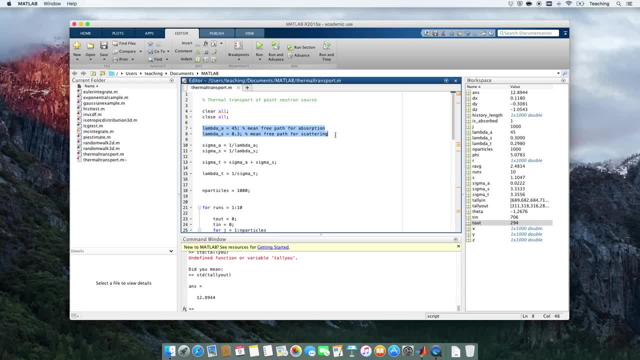 And the sophistication in those codes Arises from what sort of physical processes they treat, To what degree of accuracy they treat those processes, How the mean, free paths and cross sections are divided up In terms of energy and particle type And things like that. 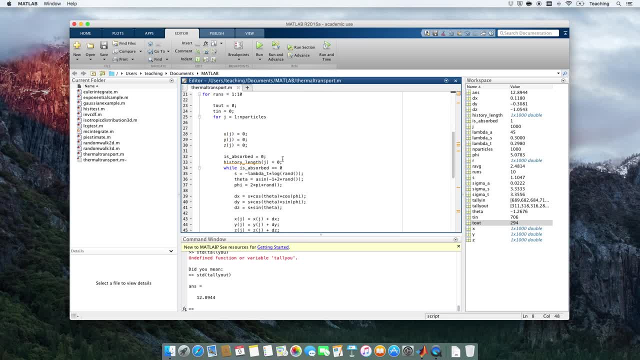 But fundamentally, All these radiation transport codes Work on this basic idea Of having a particle history Where I take a set of steps And at the end of each step I decide what to do. So there we have it: We've written a neutron radiation transport code. 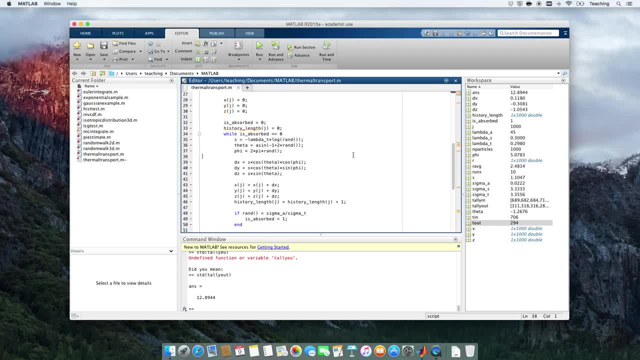 Using Monte Carlo methods from scratch, And in future videos We'll show other things we might do With that sort of calculation. 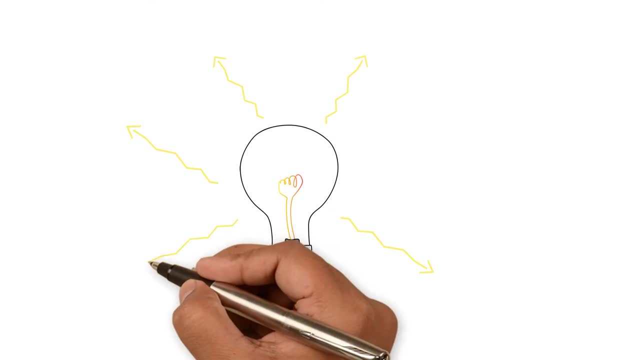 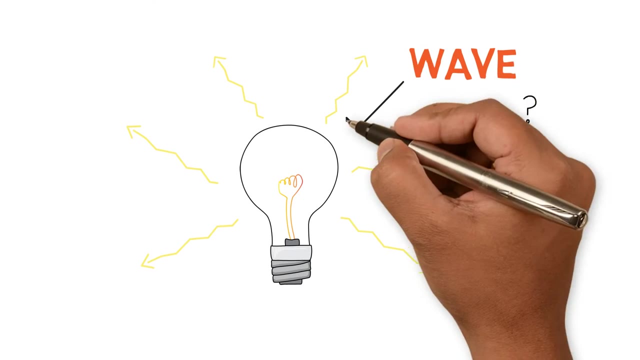 Ever wondered what light is? You can't touch it, you can see right through it. It's just there. It's probably some sort of wave. you might think after remembering all those drawings you've seen of arrows coming out the sun. Wait, no, it has to be particles, like everything else, right? 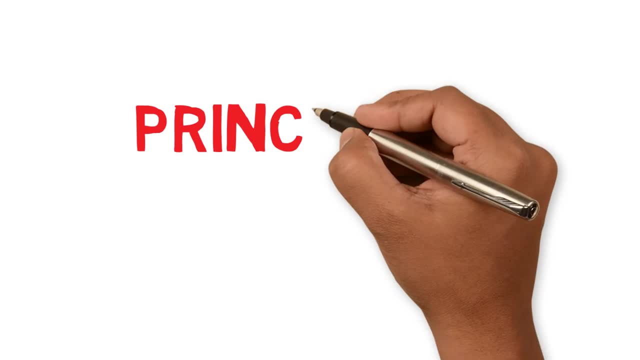 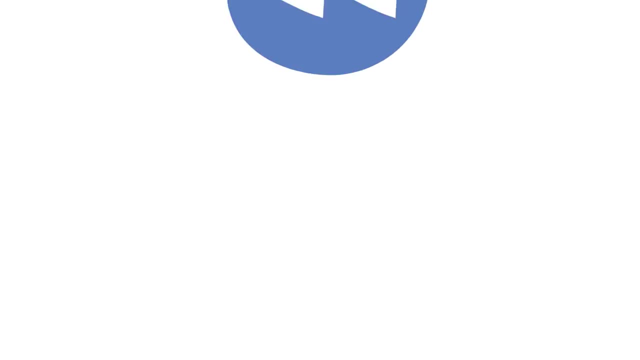 Actually, it acts like both. It's a waveacle. This phenomenon can be explained using the principle of complementarity In less than 5 minutes. hopefully, you'll understand what this concept means. Okay, let's go back a bit. The complementarity principle was first announced in 1928 by Danish physicist Niels Bohr. 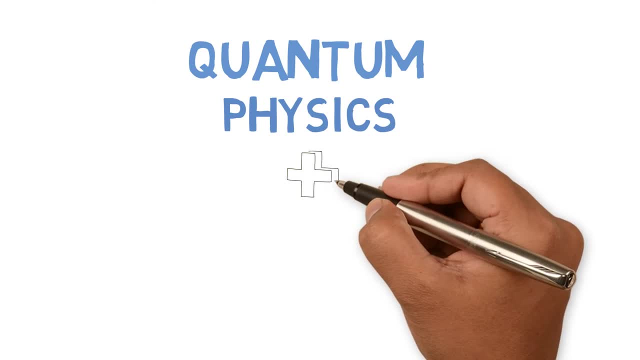 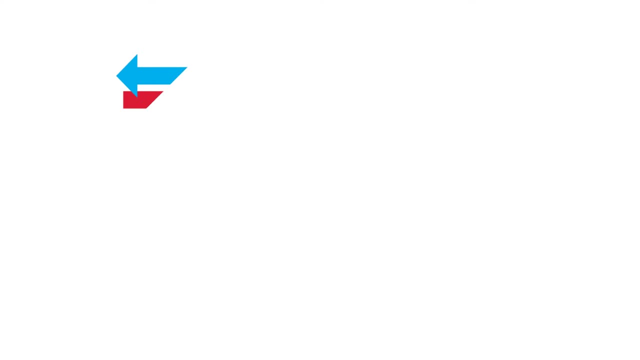 As a leading scientist in the 20th century, Bohr's most important work was applying new quantum concepts to the atomic and molecular structure. His discovery, put simply, was that objects have different properties, but these properties cannot always be seen at the same time. 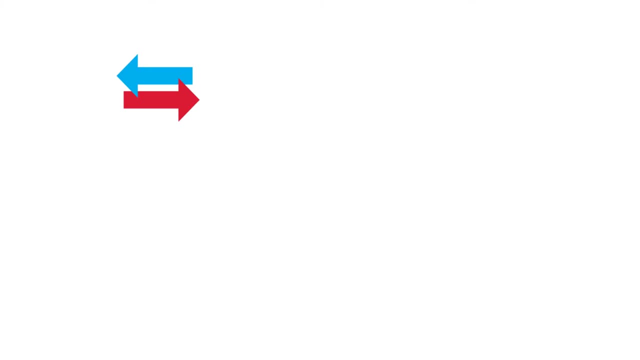 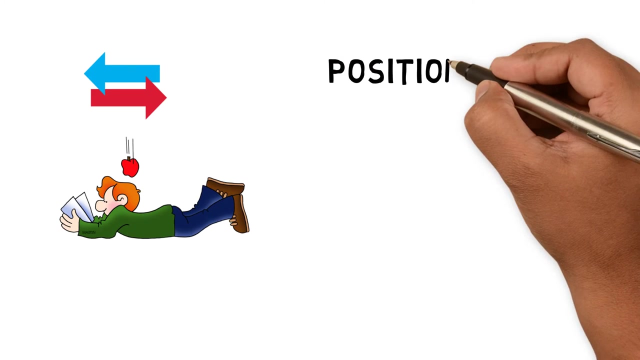 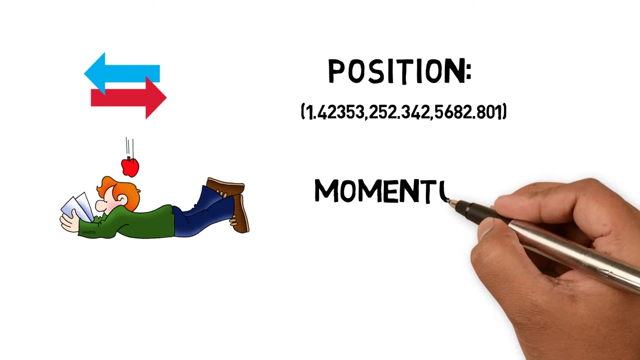 Most of these properties existed in pairs that worked in a trade-off system: Find one property and lose the other. This is perhaps one of the most important topics in quantum physics. One famous example is that of position and momentum, Originally proposed by German scientist Werner Heisenberg. the uncertainty principle states that the more precisely a particle's position is known, 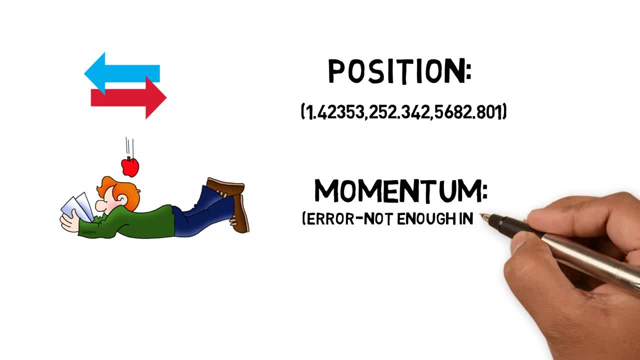 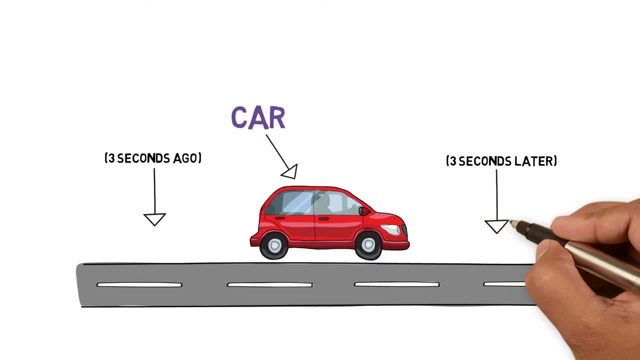 the less precisely the same particle's momentum and spin can be known. and vice versa. Imagine watching a car slowly coasting down a straight road. Well, now you can easily tell where it was and can reasonably assume it'll continue in the same direction.